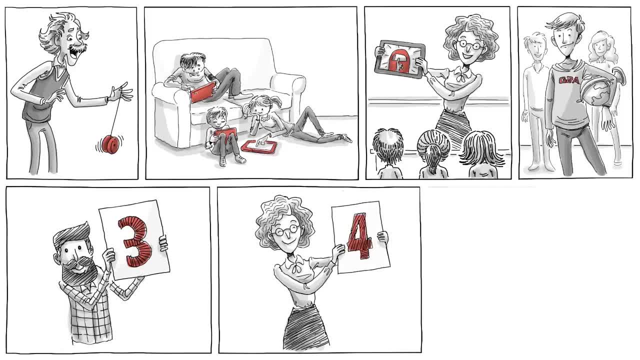 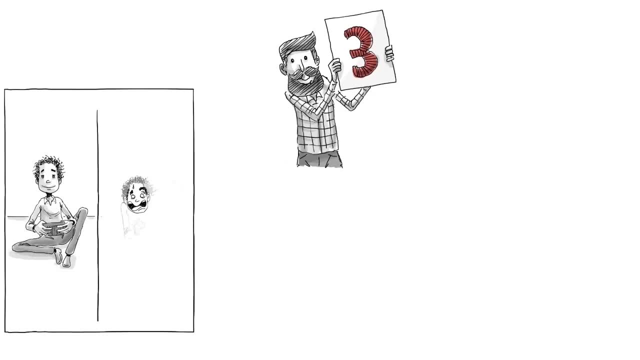 of game design: four things games can potentially teach us and five video games that are great for learning, one of which is played at Harvard Business School. First, the three dimensions of video game design. Games typically range from simple to complex. They can be played in a single. 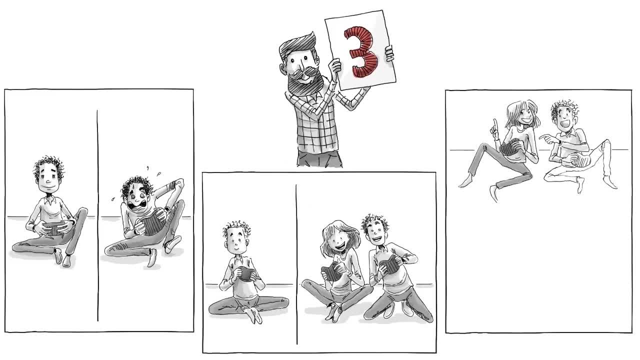 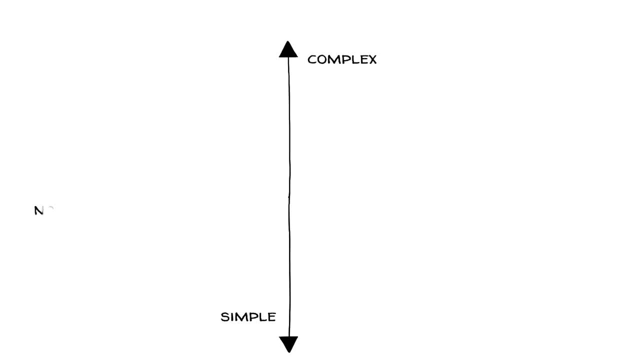 or multiplayer mode and can be played collaboratively or competitively. We can divide games along the spectrum of simple to complex and non-social to social. Simple single player games include puzzles and jump and run games Like Super Mario Complex. non-social games include the shooters like Far Cry, or simulations like 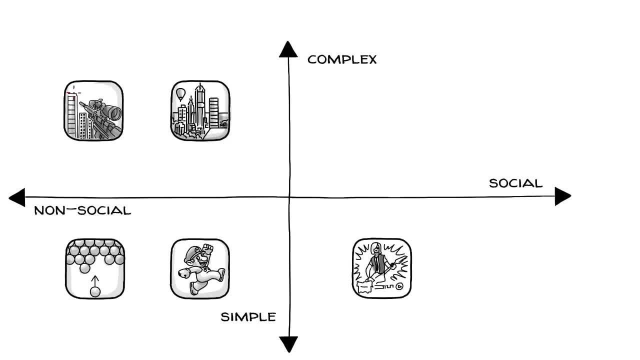 SimCity. Then there are simple multiplayer games like Guitar Hero or Need for Speed, and games that are complex and social, such as Halo, Minecraft or Among Us. Games can be competitive, cooperative or both. Complex multiplayer games are usually most effective. 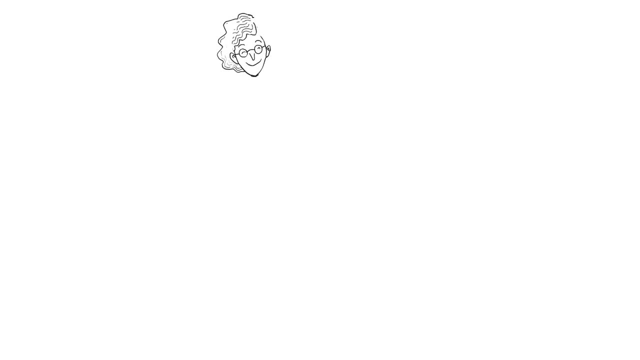 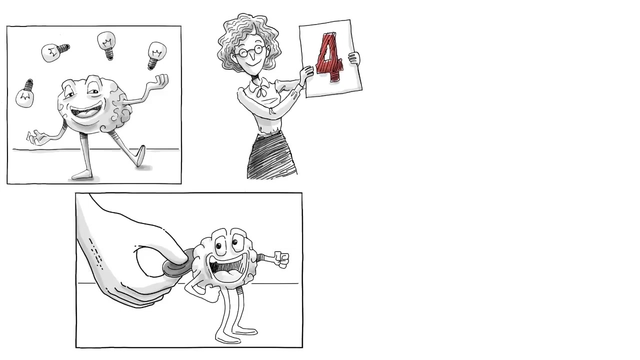 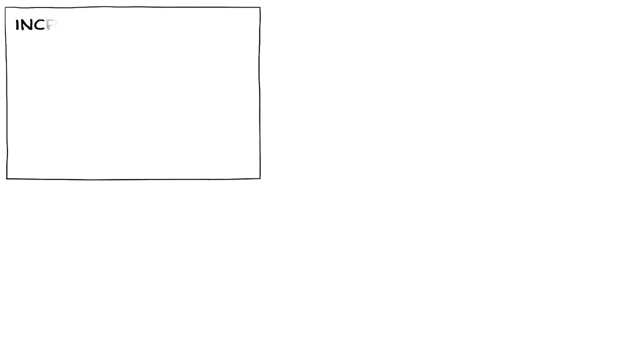 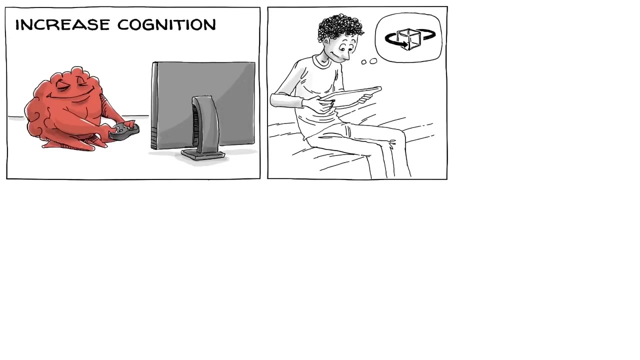 for learning. Now on to the four things games can teach us. Video games can increase our cognitive abilities, boost our motivation, make us aware of our emotions and strengthen our social skills. Games can increase cognition by strengthening particular areas of our brain. One meta-analysis showed that video games effectively teach mental. 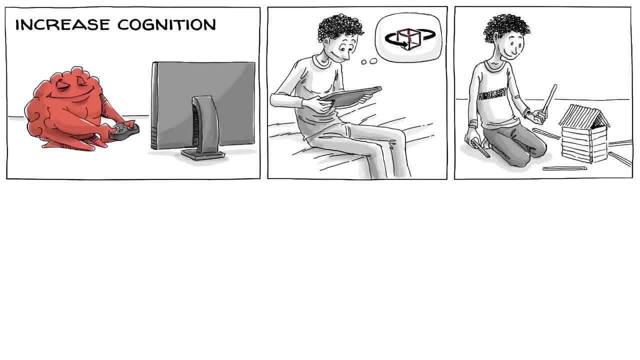 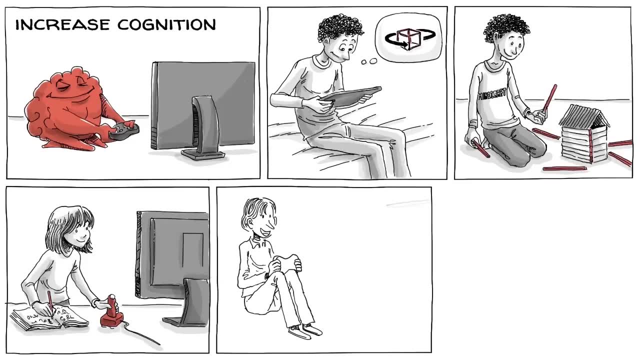 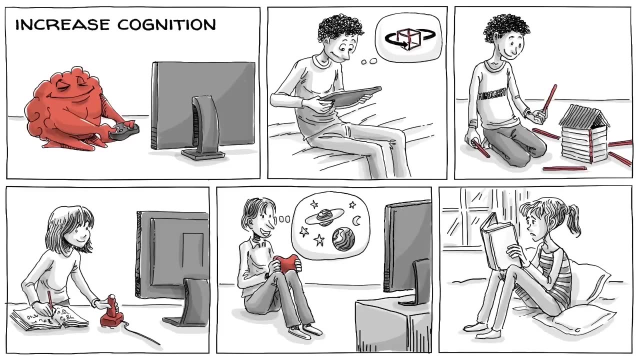 rotation abilities, and that such learning can be transferred to the real world. Logic and mathematical thinking can also be effectively learned through specific video games. Shooter games, for example, often train our understanding of relations among objects in space better than regular high school programs. Games can boost our motivation and warm us up for learning. Feedback loops that 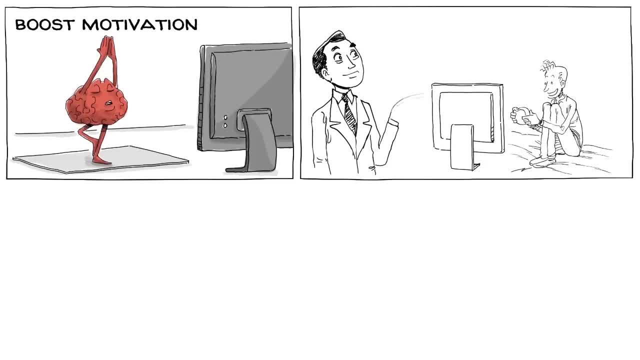 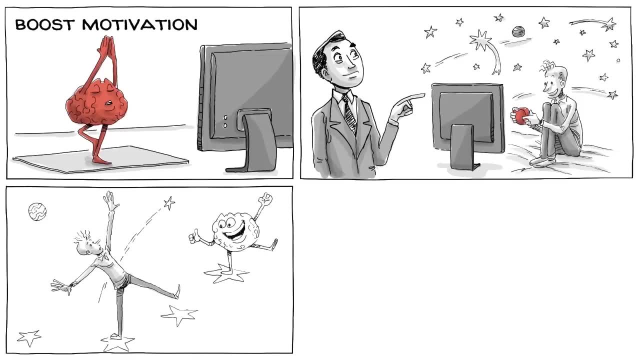 adjust to one's abilities, keep players within what Vygotsky called the zone of proximal development, And as we learn that we advance through the process of trying, failing and doing, we can develop a growth mindset. Some of the confidence we gain through games can be transferred to other. 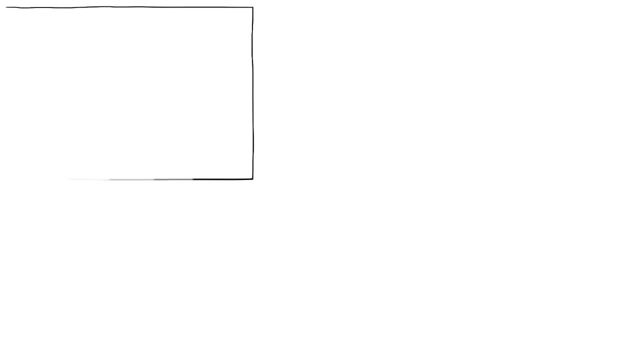 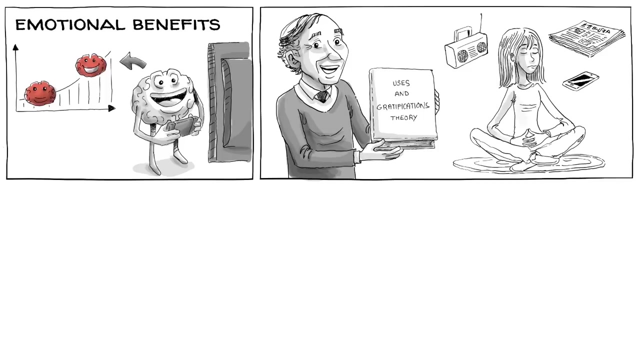 aspects of life. There are emotional benefits, and some studies report a causal relationship between playing video games and improved mood. This makes sense, being that, according to uses and gratification theory, most of us seek diverse forms of media to manage our mental state. 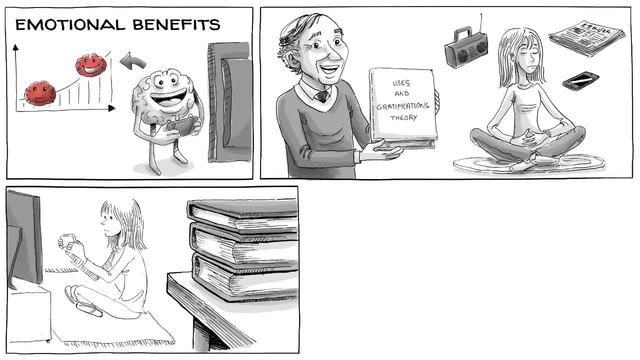 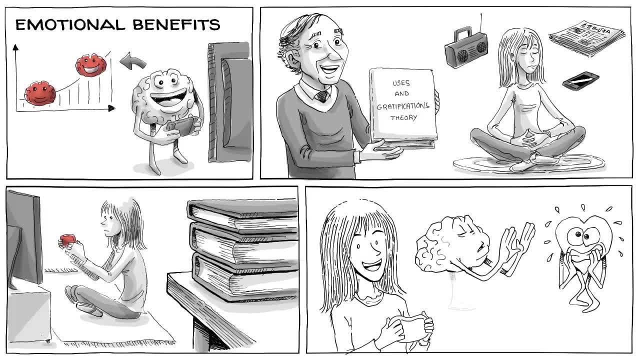 Putting the books aside for a short game break can therefore enhance our emotional state. One study reported that gamers often experience high levels of stress and, as a result, learning to manage their emotions. There can be social benefits as we form new relationships. 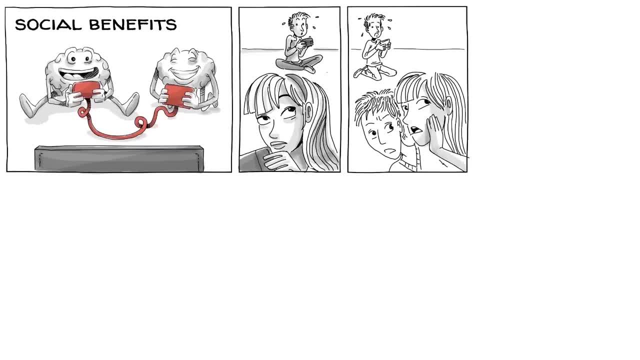 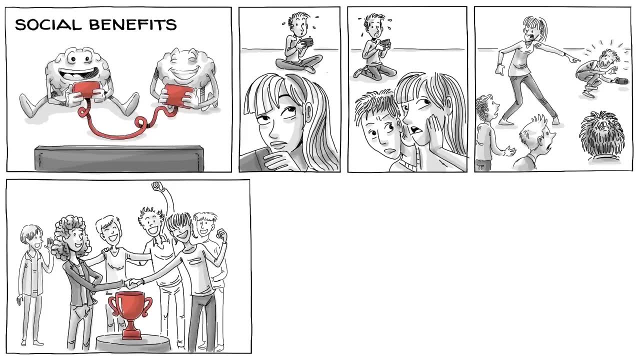 In some games we need to learn who to trust, how to communicate and when to take the lead. Video games that are designed to reward cooperation promote pro-social skills particularly well. One longitudinal study found that children who played more pro-social games at the beginning 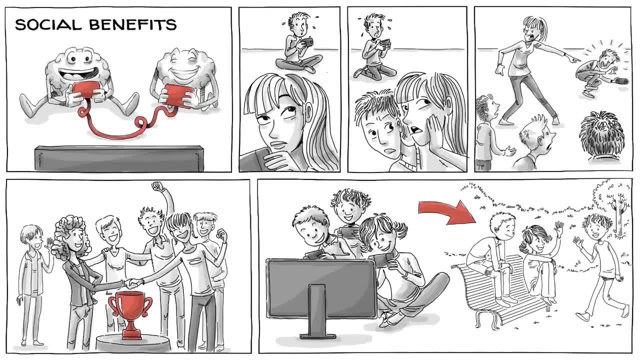 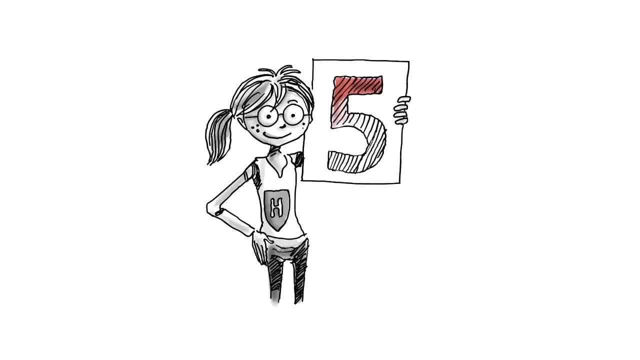 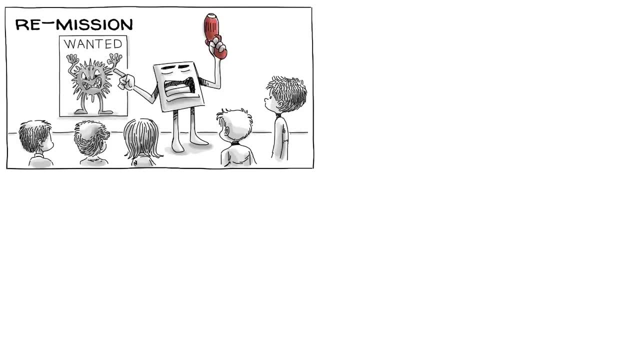 of the school year were more likely to exhibit helpful behaviors later on in the year. Finally, let's look at five games that deliver powerful learning experiences. Remission is a video game that teaches sick children how to deal with cancer. In the game, the children control a nanobot that shoots cancer cells and manages the 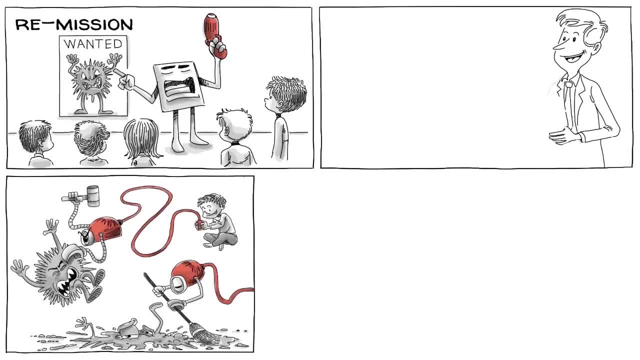 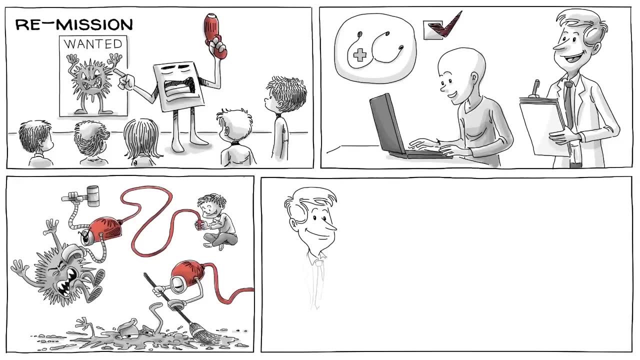 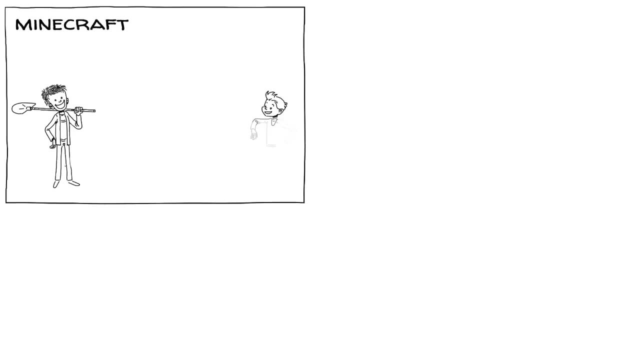 side effects of the treatment. A randomized control trial showed that children who played Remission significantly increased adherence to the treatment protocol and cancer-related knowledge. The game has since helped hundreds of thousands of young patients. The game Minecraft promotes creativity, collaboration and problem solving. through trial and error, Players build their own world and 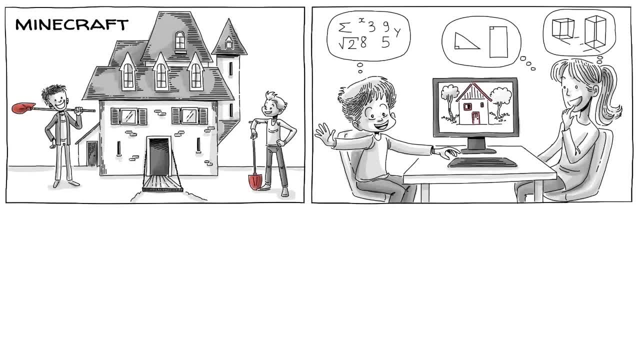 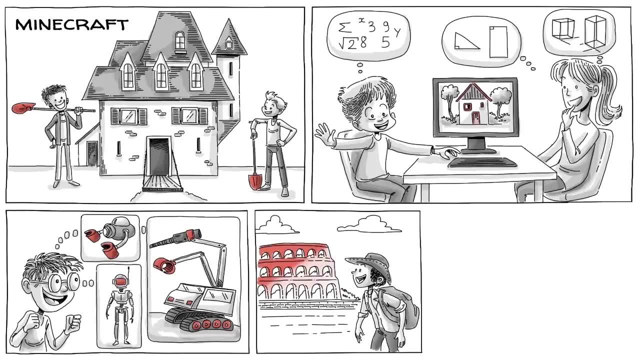 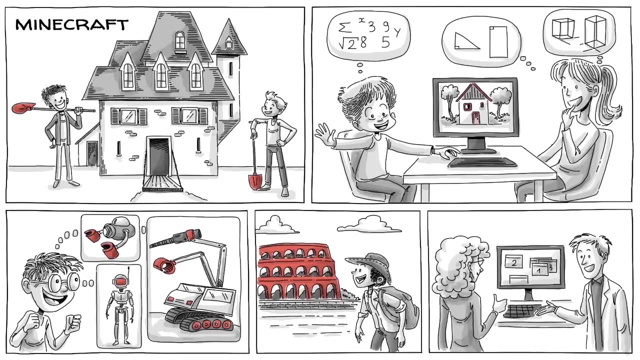 alongside, apply math and learn about shapes and geometry. Some do electrical engineering and build machines that run in the virtual world, and others explore human history. Its Education edition gives teachers special control and access to a wide catalog of lessons: Demo, Demo and Demo. 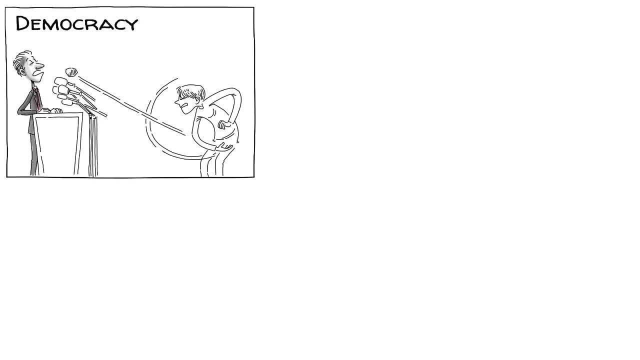 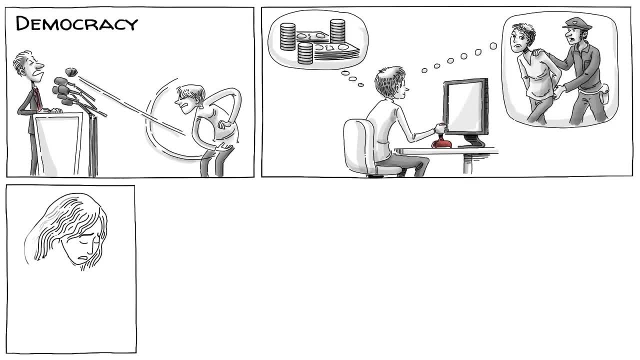 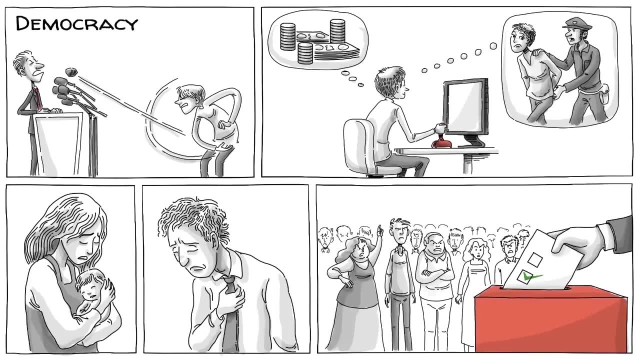 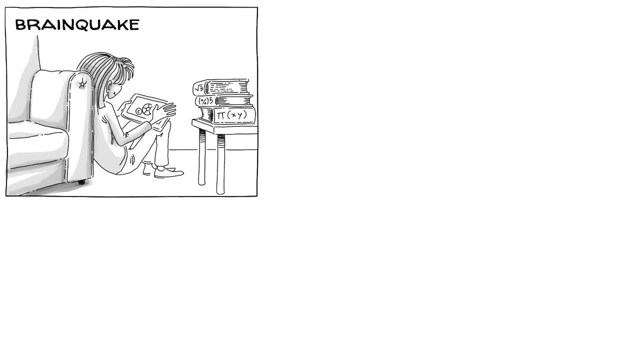 and discover how policies affect real people. They have to deal with difficult issues like immigration and unemployment and then still try to win the majority support in the next election. The app BrainQuake allows students to learn math in a playful way and without using symbolic language. 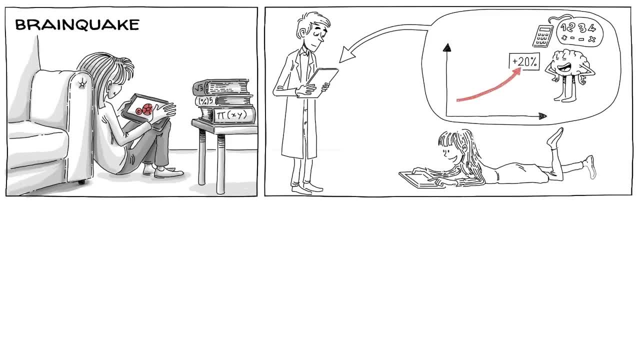 Controlled experiments showed improved math scores by 20% when third graders play the game for just 10 minutes per day, three days a week for a month. The game was developed with the help of the popular math teacher Keith Devlin. Its education edition allows teachers.